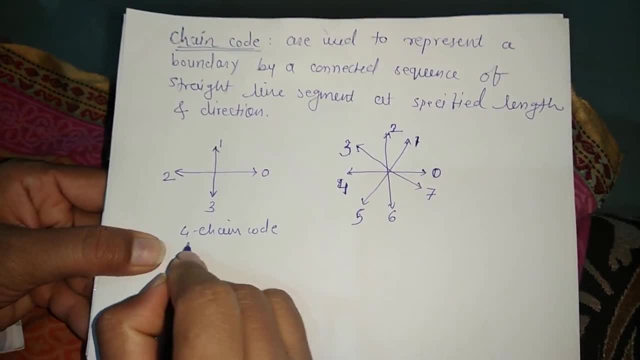 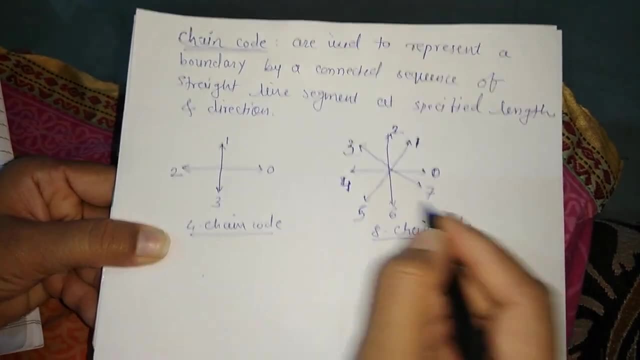 up, down, left, right. So you have to use this 4 chain code or you can use the 8 chain code when there is a boundary region where the diagonal points are being present in the shape. 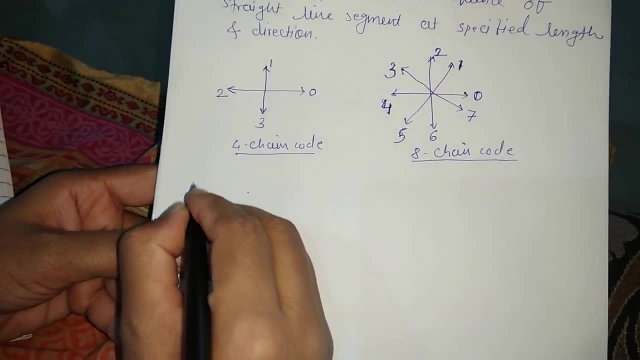 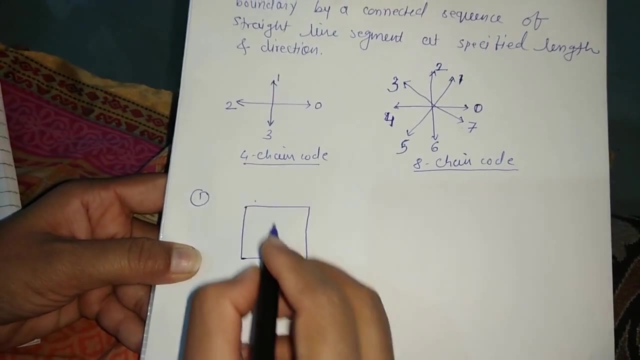 We'll take a simple example. Here is simple shape is given. It is like this. You have to start with some origin. So direction is this. It is moving. We have 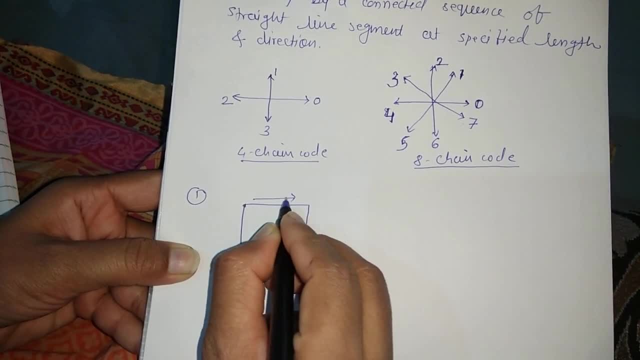 considered this is the origin. In this direction it is moving towards right. The code is 0. Next at reaching at this point it is moving 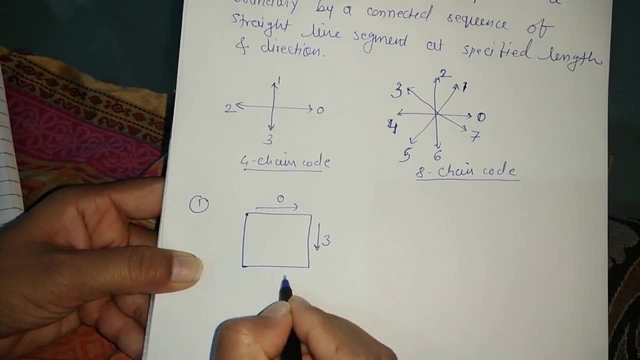 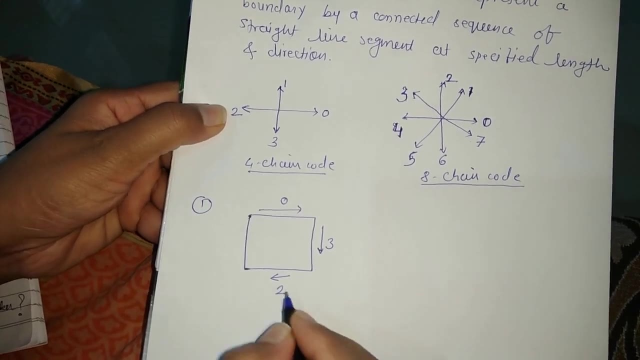 downwards. So code is 3. At this point then it is, because we have to reach towards the origin. So this left, the left is 2. Then it is moving upward. For upward it is 1. So 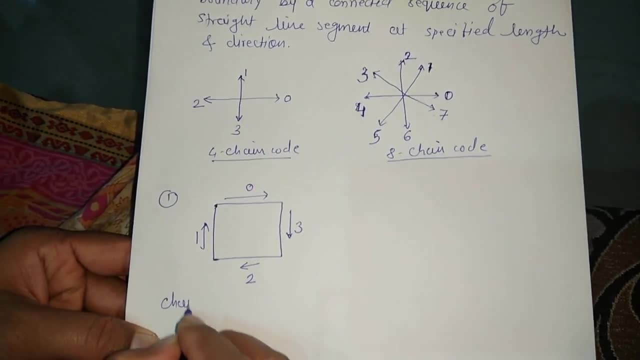 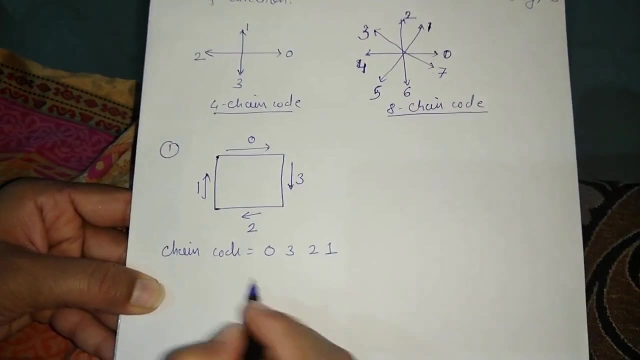 we'll specify the 1. So what is the chain code for this? What you have to, 0, 3, 2 and 1. So this is your first chain code. Then you have to find out the difference. So you 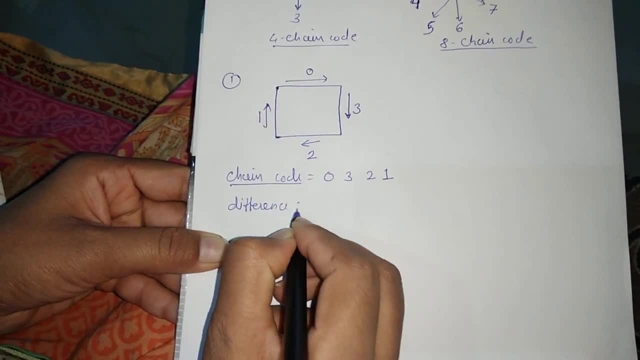 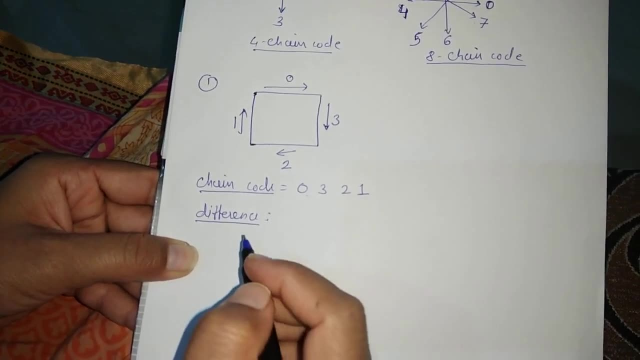 out the difference how we will going to find the difference you need to subtract this chain code in anticlockwise direction let's say you 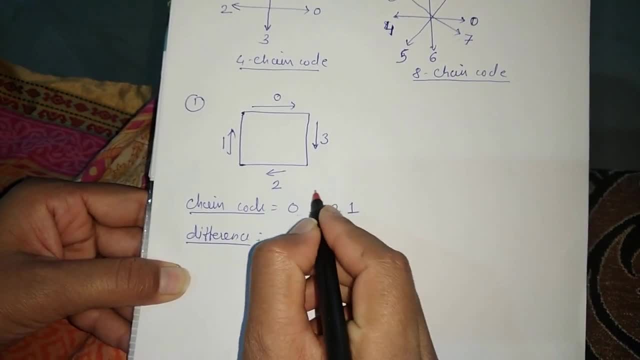 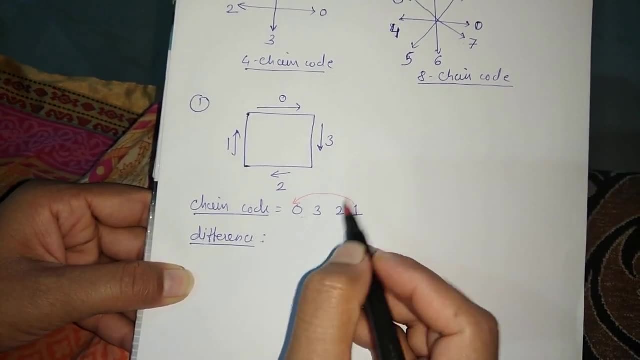 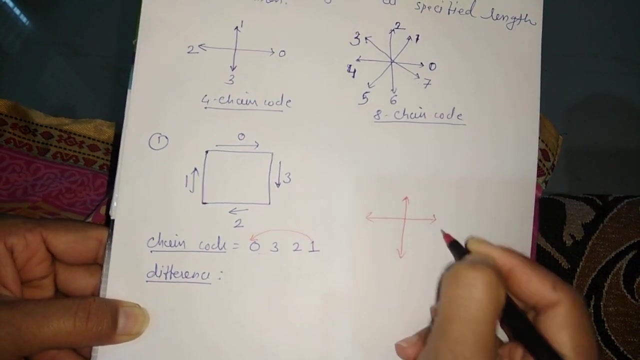 have to first you have to subtract this one from the zero in anticlockwise direction not going to do the numerical subtraction but you have to use this fourth chain code let's say this is your fourth chain code is given that is 0 1 2 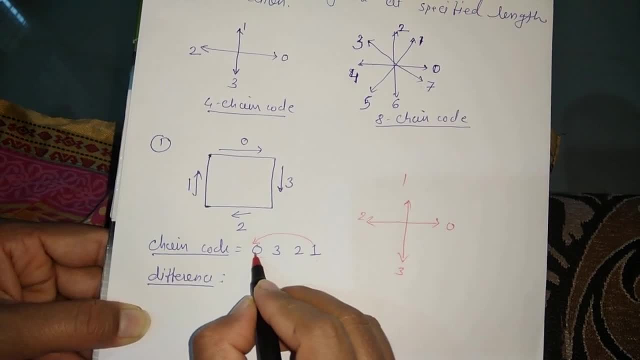 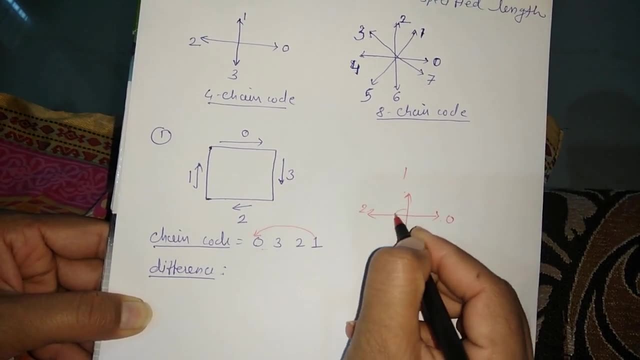 and 3 so 1 minus 0 first chain code so how you will going to 1 minus 0 you have to move anticlockwise this is 1 and this is 0 so you have to move anticlockwise and 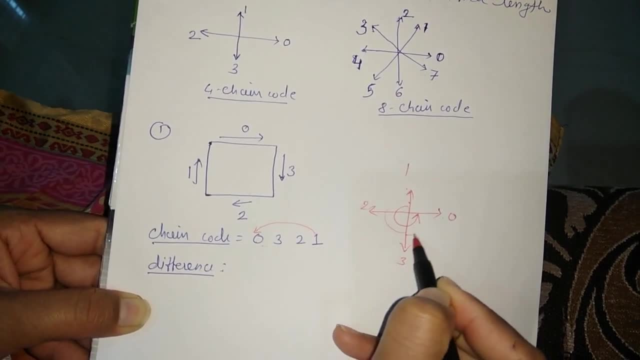 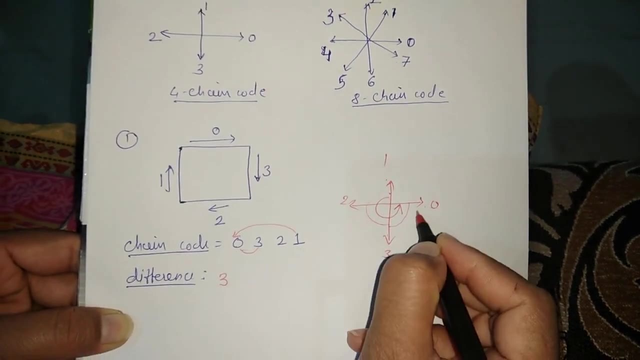 the distance is this is 1 this is second this is third so difference is 0 next is 0 3 0 3 so we 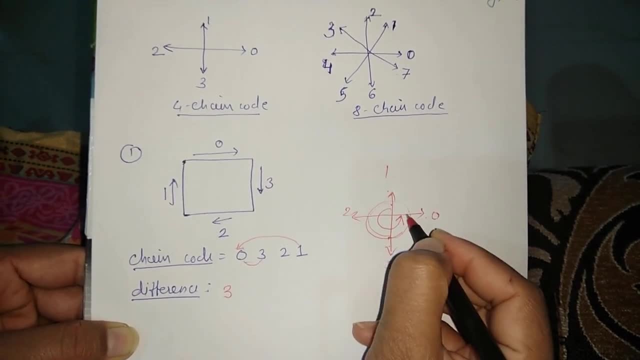 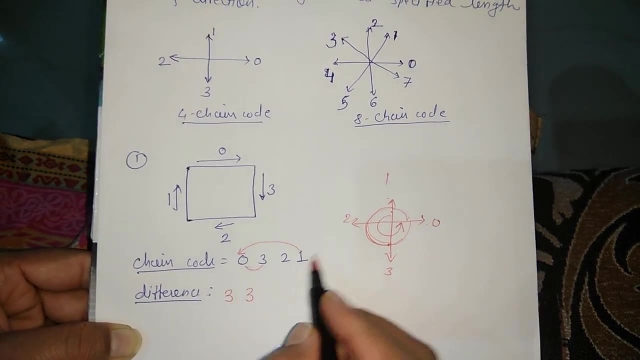 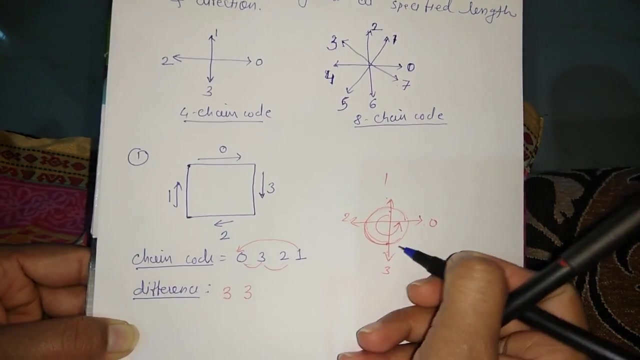 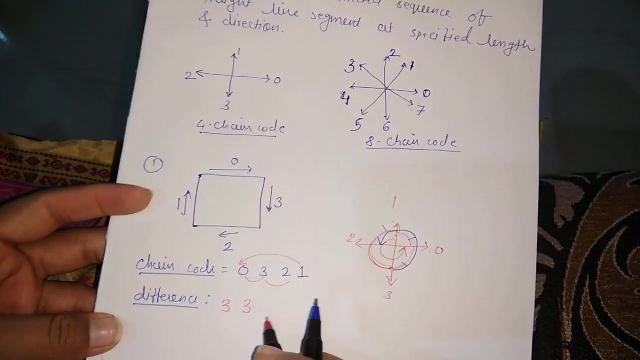 have to move in anticlockwise direction till 3 this is 1 2 and 3 so this is 3 then next is 2 sorry 3 minus 2 3 and 2 so you have to move in anticlockwise direction from 3 to 2 to like this so this is 1 2 and 3 the difference is 3 the next is 2 1 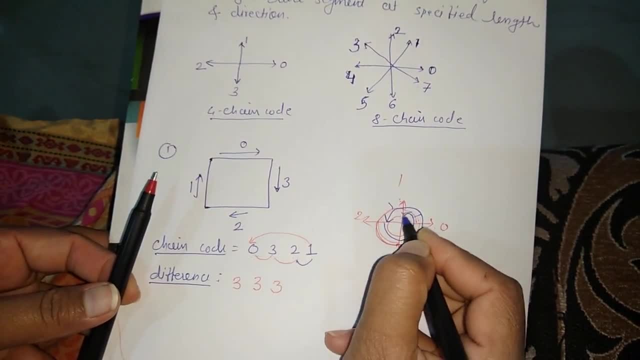 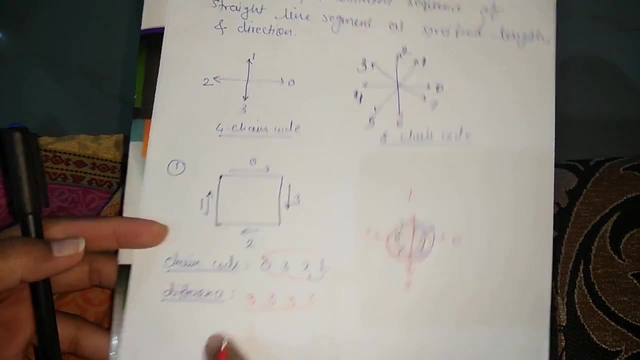 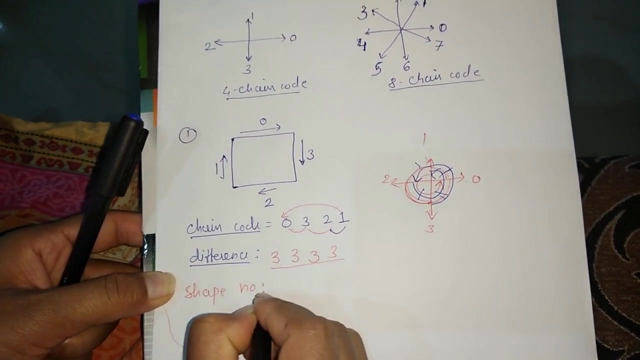 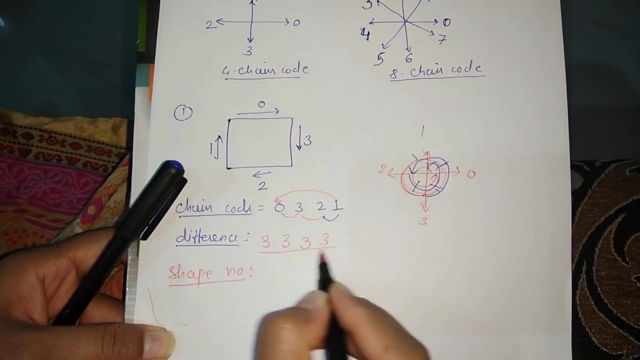 so in this 2 and So you have to move in an anti-clockwise direction the 1, 2 ,3 the difference is what you have got the difference three 3 3 so what you have got the difference 3 3 now the next is you have to calculate the shape number so how we're going to identify the shape number you have to identify the lowest difference value in this here is a lowest difference value is 3 so 3 and you have to copy the last values from here so 3 so 3 and next you have to copied all the three numbers» once again let me call in the number first. 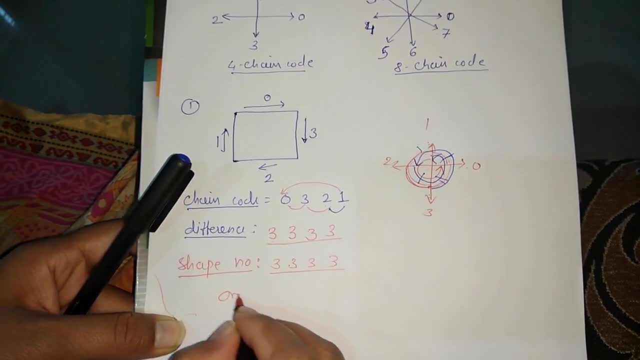 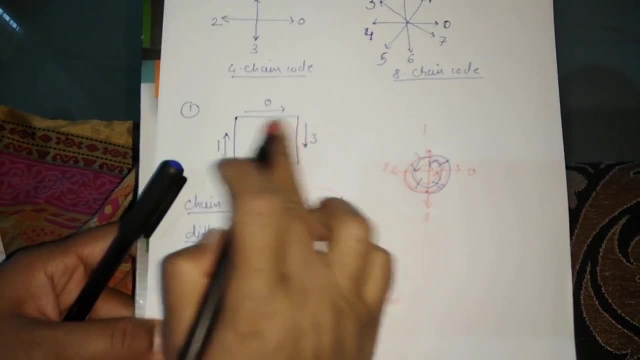 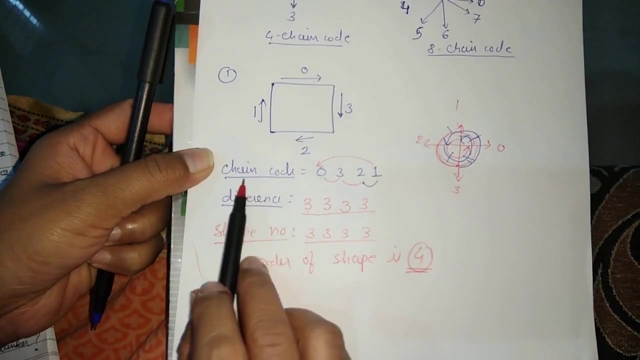 as it is so this is your shape number and the order of shape is four one two three and four so this is the simple for this given simple shape you have to identify 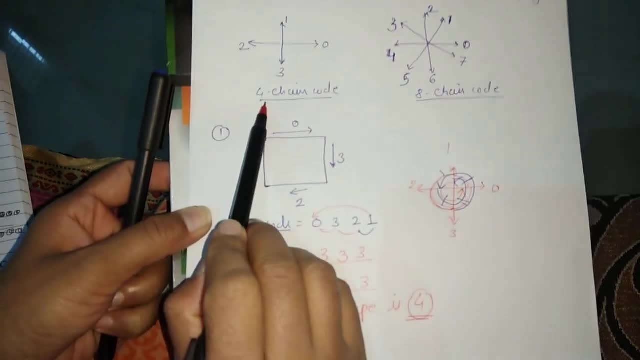 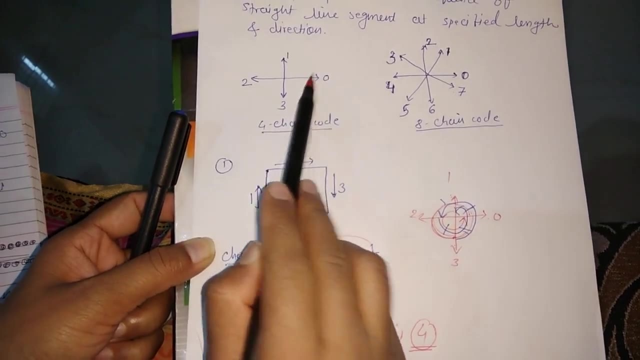 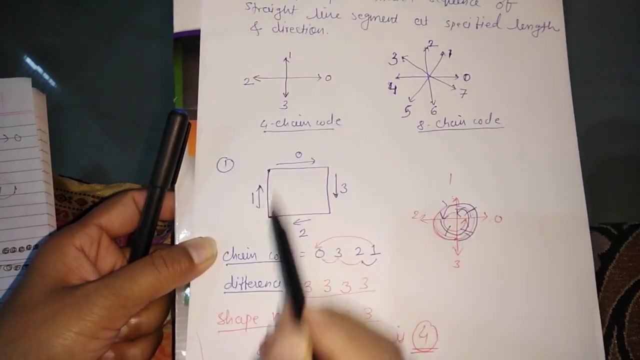 the chain code for identifying the chain code you have to use if in problem if asked with the four chain code you have to simply use this the shape you have to identify the direction of the shape if it is moving right zero downward is three left two upward one then you will get the chain code 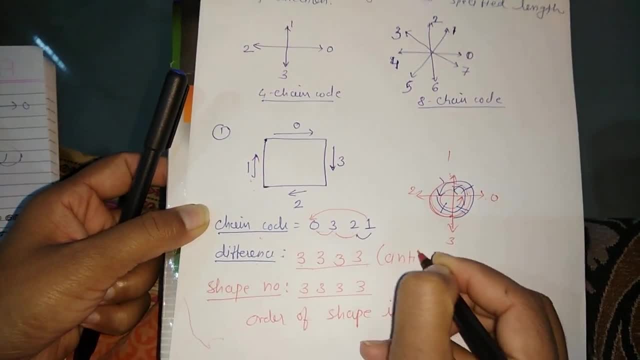 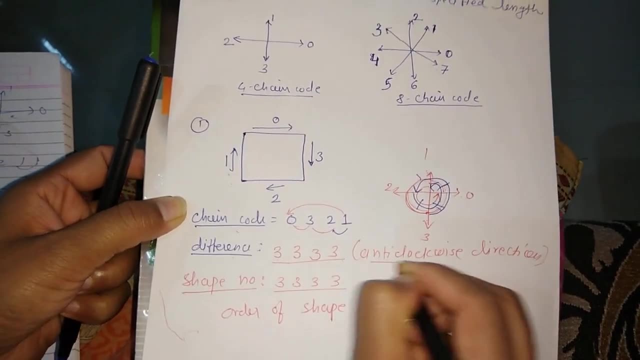 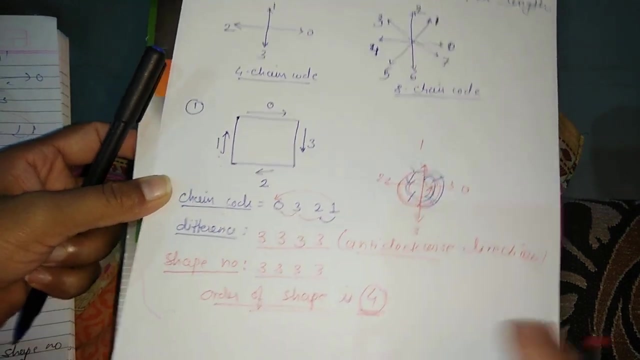 then difference difference find out in anti-clockwise direction and last one is shape number and then you will get the order of shape is four we'll see a next example 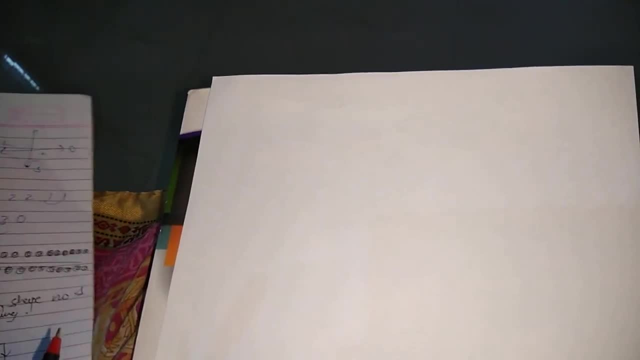 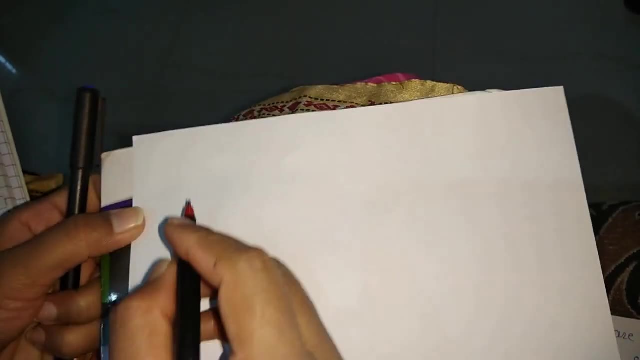 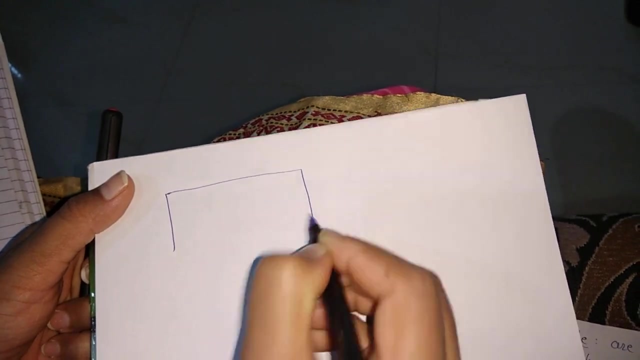 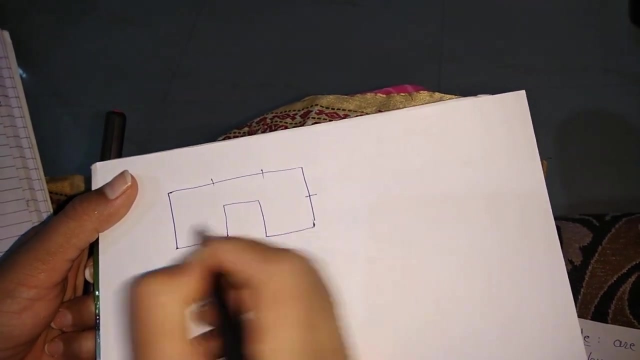 so the question is given as the problem or the shape is given as like this you can see here so this is worst first half second third 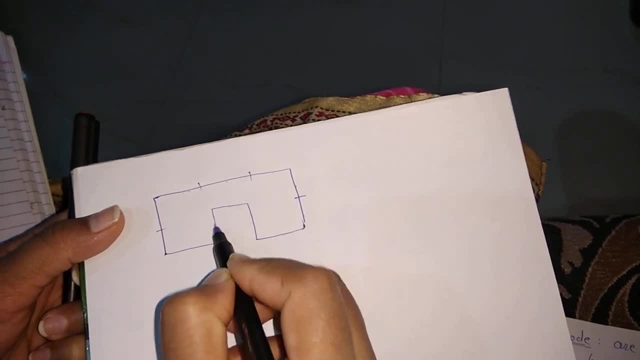 fourth fifth sixth seventh eighth ninth tenth eleven and twelve this is moving in this direction 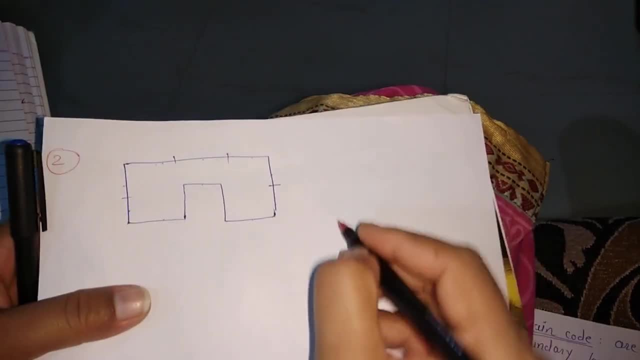 at side you have to just draw this fourth chain code we are solving using fourth chain code this 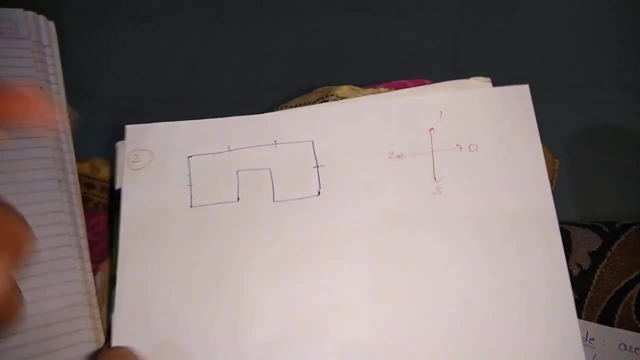 is zero one two and three so simply you can write here itself this is origin we are considering so 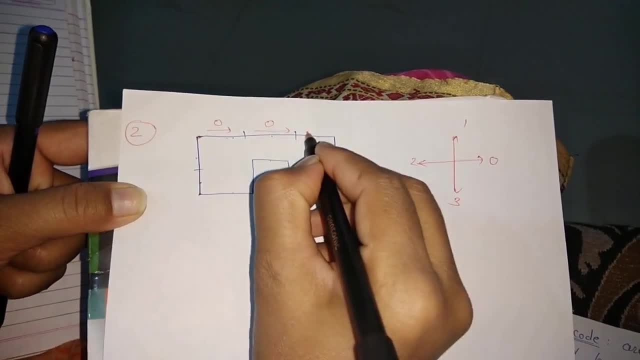 this is zero this is again right zero this is again towards right zero 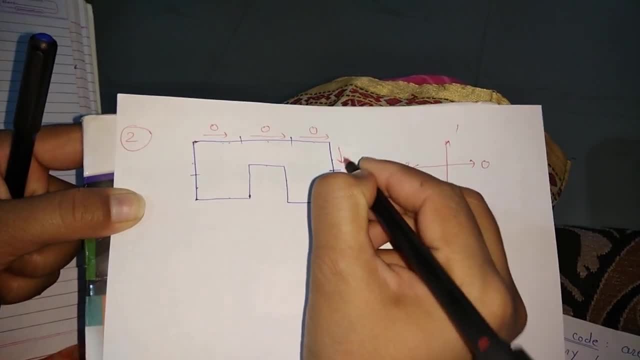 then it is moving downward the downward value is three down water values three then 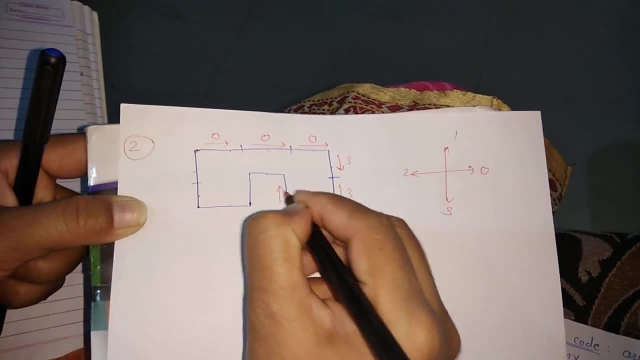 it is moving left left is two moving upward value is one 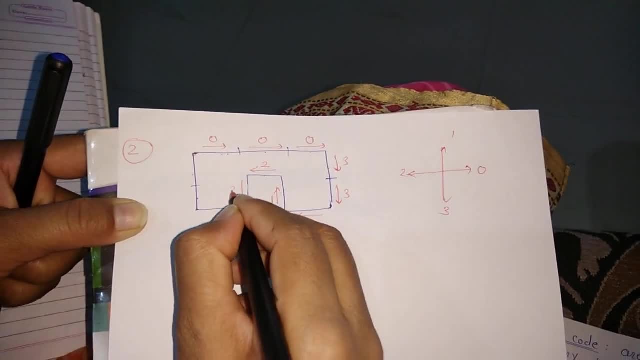 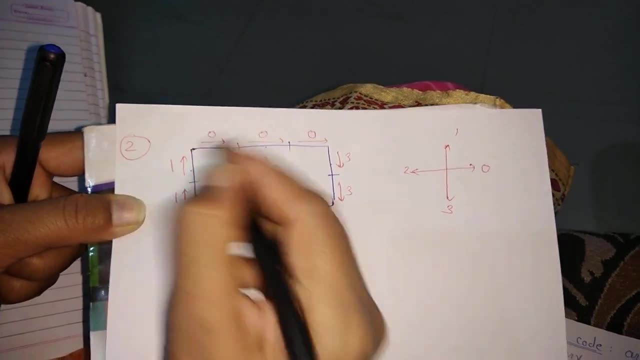 moving left value is to moving downward value is three moving left it is 2 upward 1 upward 1 you have got the chain code value using for chain code 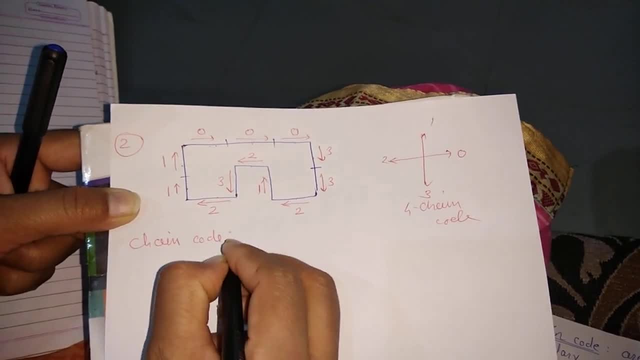 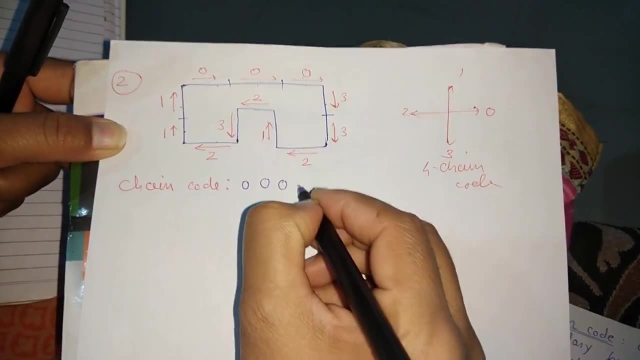 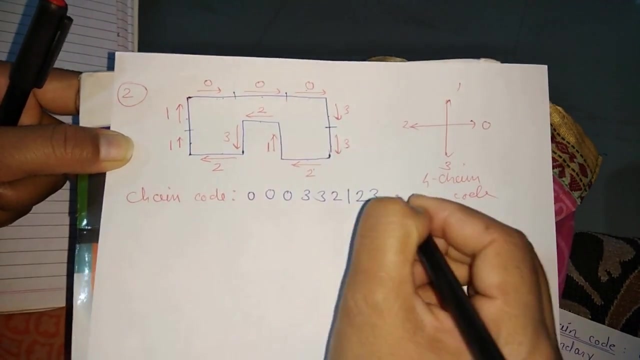 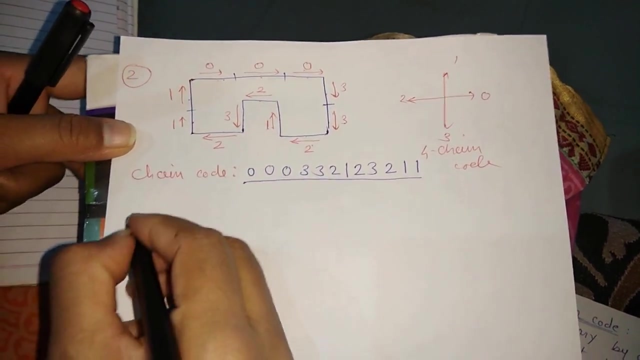 So you have to write the chain code. So what is your chain code is 0, next 0, 0, 3, 3, 2, 1, 2, 3, 2, 1 and 1. So this is your chain code. The next step is you have to find the difference. 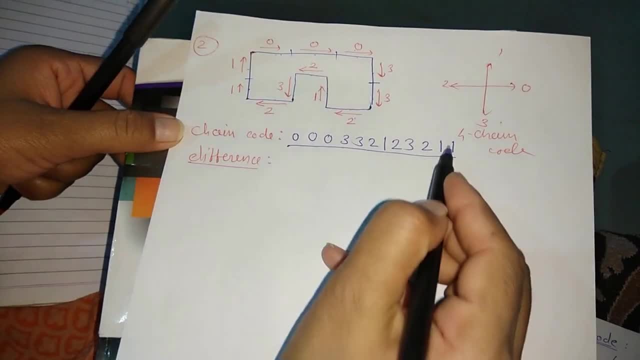 How you are going to find the difference? You have to move in anticlockwise direction and then find out the difference. 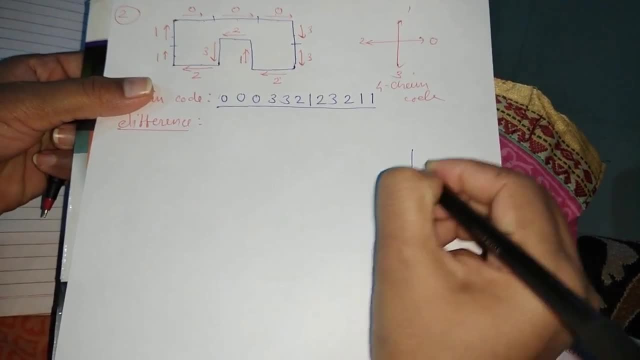 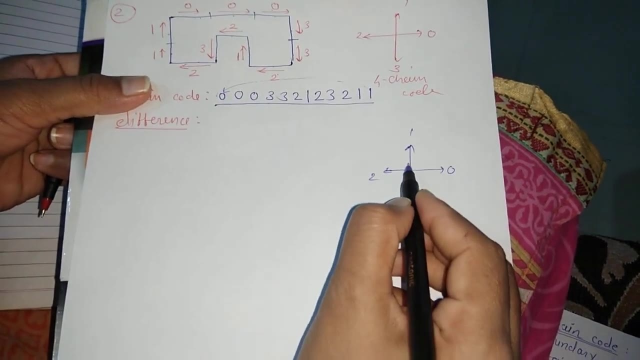 So you have to use this. 0, 1, 2, 3. 1 minus 0, 1 minus 0 anticlockwise. So 1, 2 and 3. 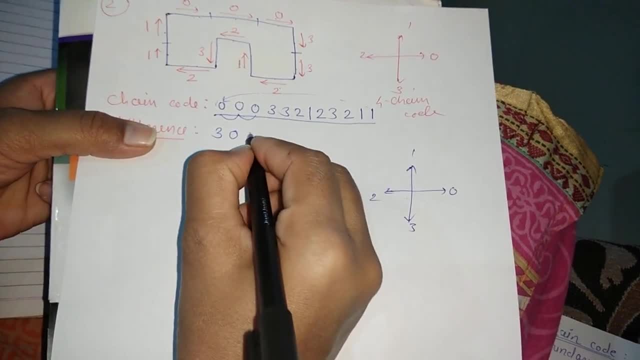 Then 0 minus 0, it will be 0. 0 minus 0, 0. 0 minus 3, 0. 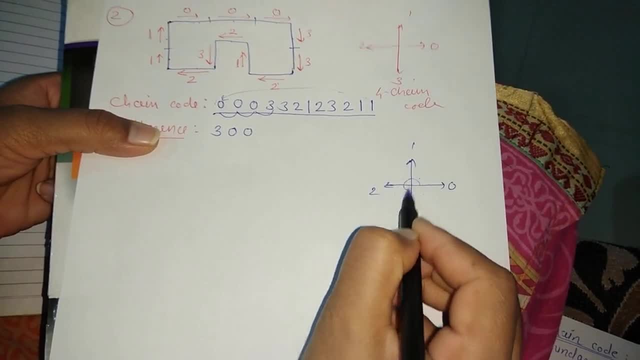 0 to 3 anticlockwise, you will move like this. So 1, 2 and 3. 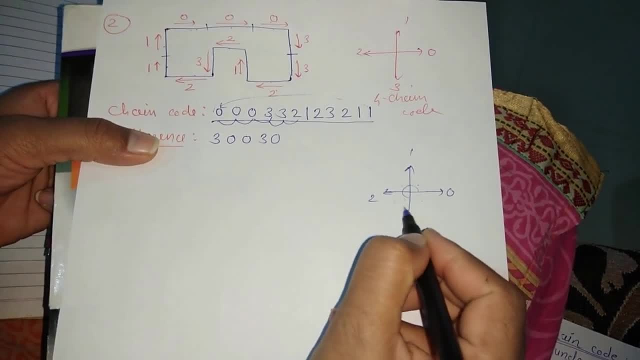 3 minus 3, 0. 3 minus 2, 3 minus 2. So 1, 2 and 3. 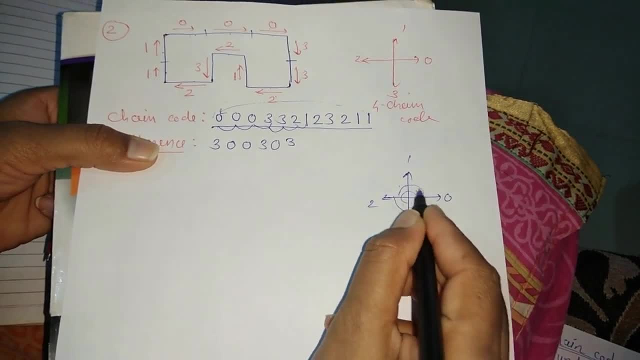 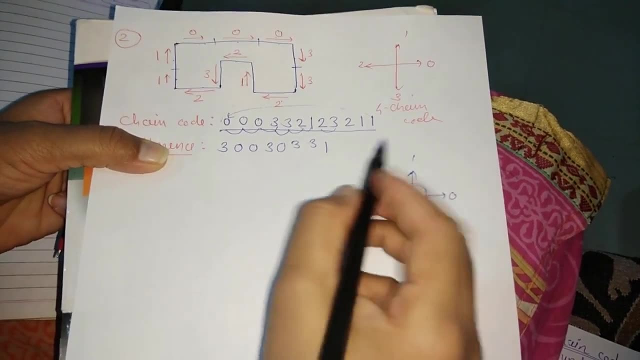 2 minus 1, 1, 2. 2 minus 1, 2, 3, 2, 3. Anticlockwise, so this is 1. Next is 3, 2. 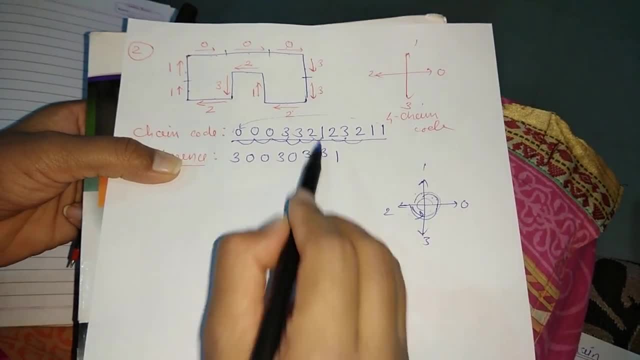 Sorry, 2, 1. Then 1, 2. 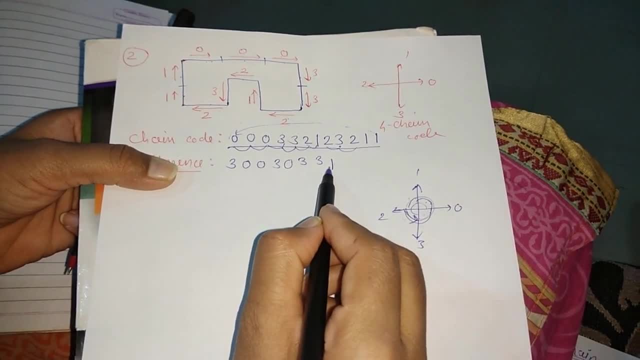 1, 2 is 1. Next is 2, 3. 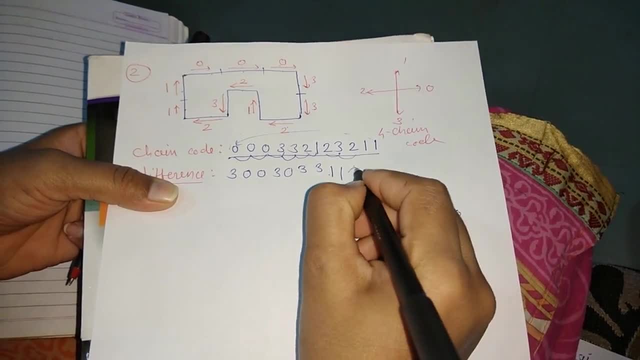 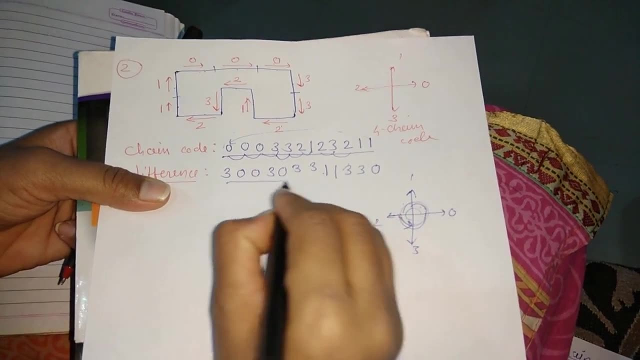 1, then 3, then 3, then 0. Okay, you will got this difference. So you have to use this value for this. 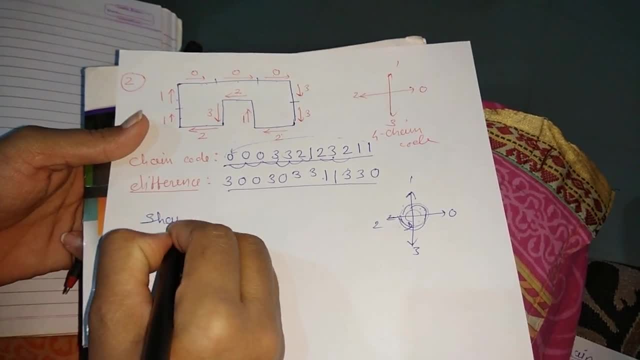 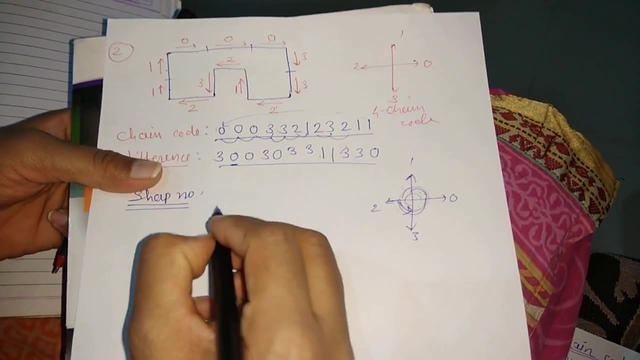 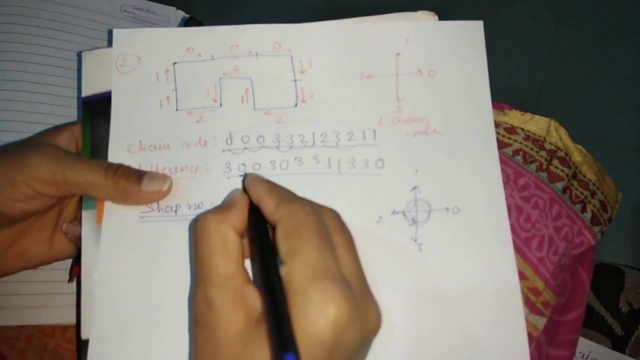 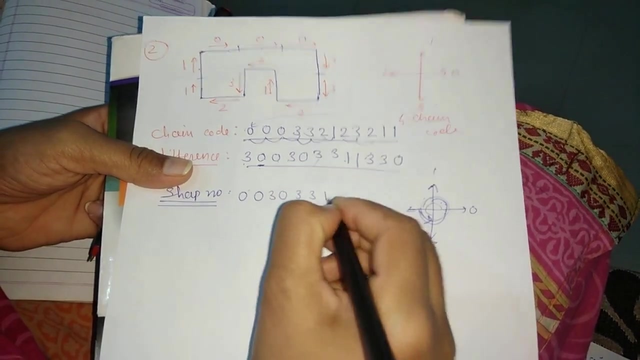 Then you have to find out the shape number. So how you will going to identify the shape number? You have to take a lowest value from this. The lowest value, you have to start with this. The next lowest value in this is 0. So you have to start with this 0. Next 0, 3, 0, 3, 3, 1, 1, 3, 3, 0. And then you have to find out the shape number. So you have to find out the shape number. 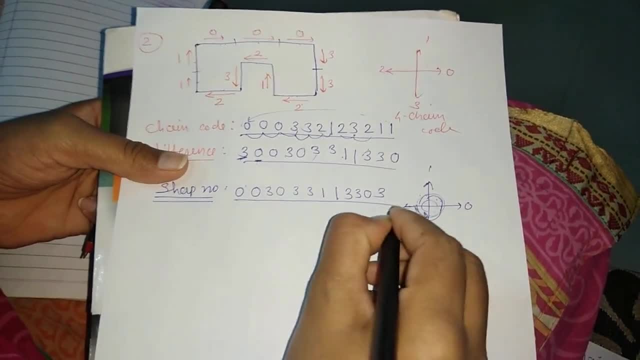 And the last remaining is 3. So this is your shape number. 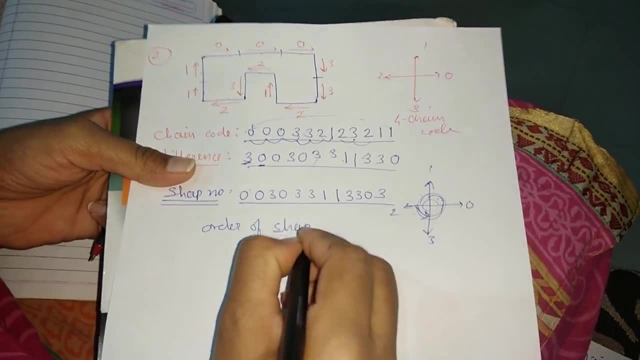 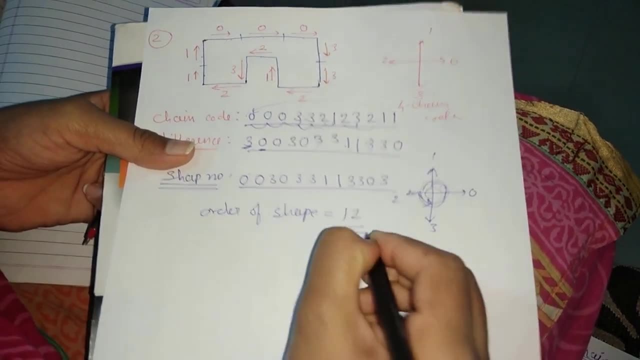 And the order of shape is 1, 2, 3, 4, 5, 6, 7, 8, 9, 10, 11, 12. The order of shape is 12. Or you can identify from this one. So 1, 2, 3, 4, 5, 6, 7, 8, 9, 10, 11, 12. 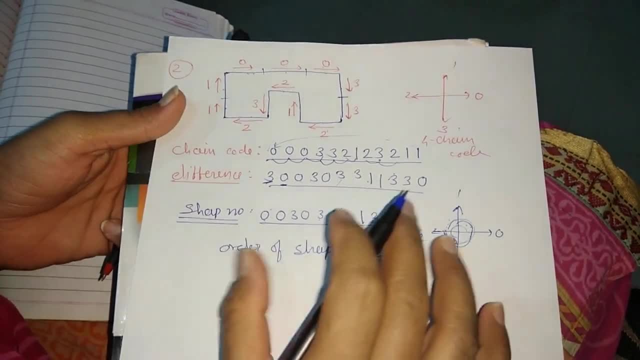 So order of shape is 12. So this is the way to find out the chain code. Then difference. 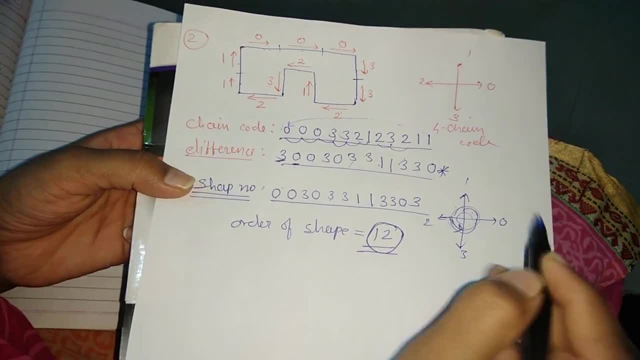 Just keep in mind anti-clockwise direction. Find out the difference. 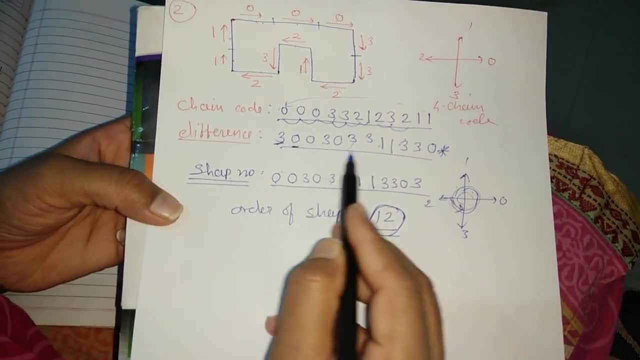 And the shape number, you have to take the minimum value. Start with that minimum value. And the remaining value you have to append at the last. 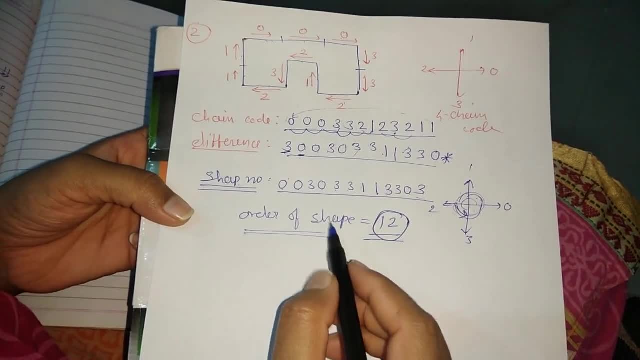 And then you will get the order of shape. So this is all about chain code. Thank you. 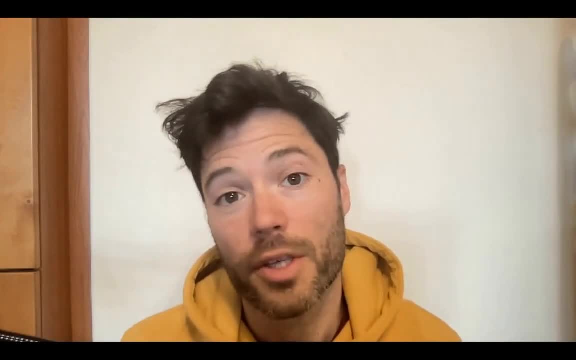 DeepSeek Coder is a new model that has been released by researchers in Beijing. It's outperforming CodeLama on a number of benchmarks. Perhaps more importantly though, 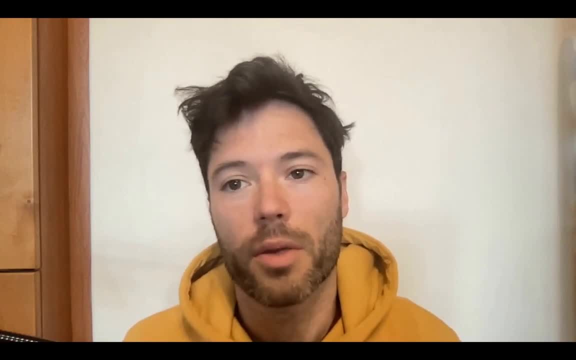 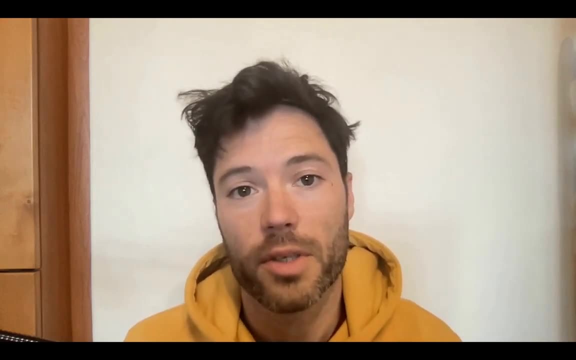 it's a very permissively licensed model, which means it can be used in an open source and commercial way without having any limitations, including limitations like Facebook's Lama, 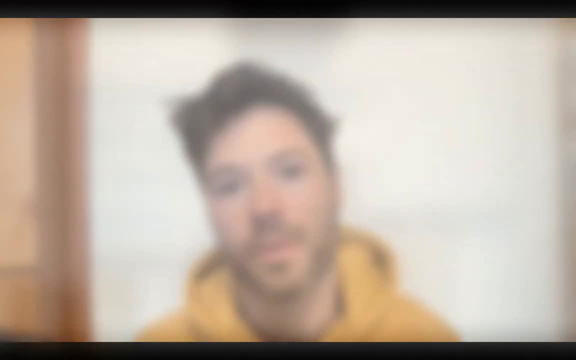 which does not allow you to train other models with it. For agenda, I'll give you an overview of the model. It comes in 1 billion, 7 billion, and 33 billion sizes. I'll talk through the prompt format, which is a little 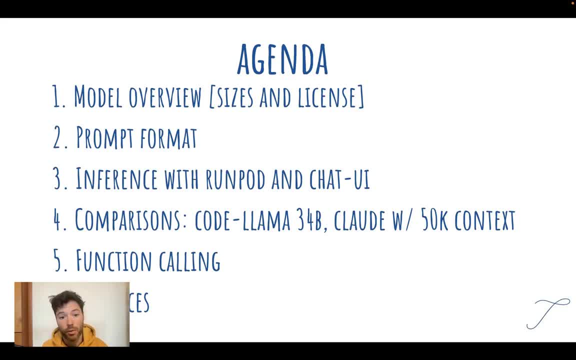 different than the Lama model. Then we'll go through inference using RunPod, which is inference on a GPU. I'll show you chat UI briefly, a chat interface. Then I'll get into comparisons with